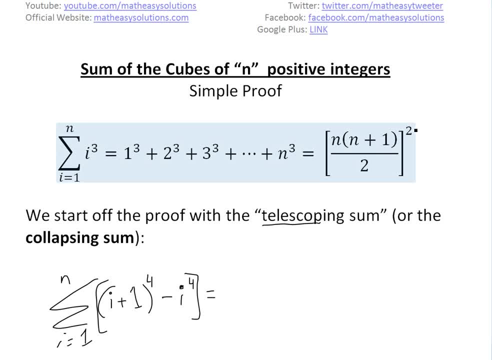 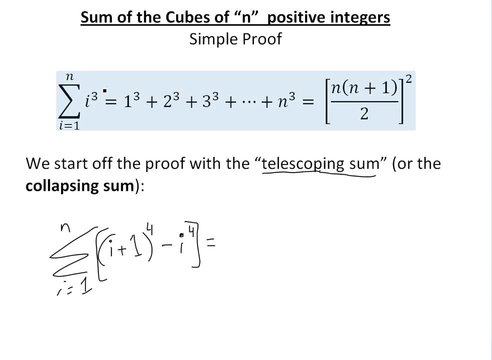 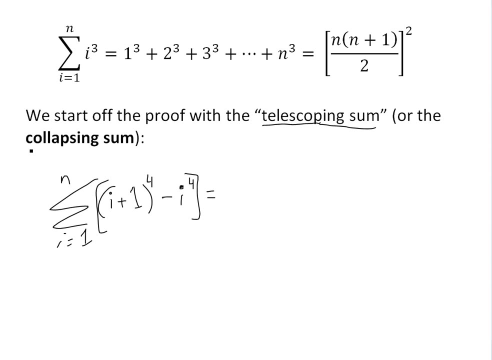 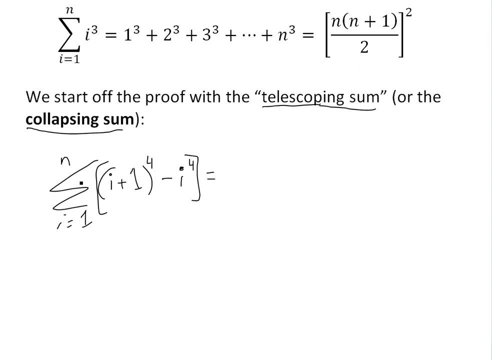 This sum is going to equal to n times n plus 1 divided by 2, all to the power of 2.. And now we're going to start off with this telescoping sum which I showed before in the squares video. It's just a useful tool. Before I had it to the power of 3 here, Now I'm going to do a power of 4.. It's useful because it collapses. It's usually called the collapsing sum And then you can use it to prove this And I'll show you what it is again. So basically, you have this one here. Sigma i is initially 1 up to n of i plus 1 to the power of 4 minus 2 cubed. 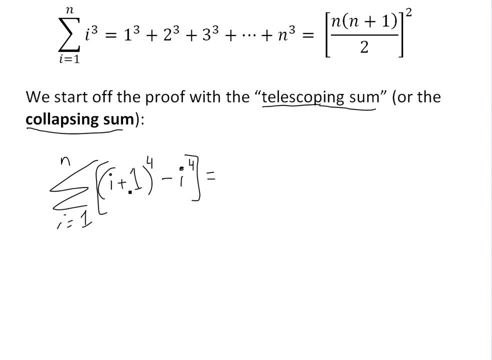 Minus i to the power of 4.. And if you write this out, Remember this one is just going to be 1 greater than whatever i is. If i is 1, it's going to be 2.. So we're going to have 2 to the power of 4, minus 1 to the power of 4 in bracket, And then plus Now the next term is going to be a 2.. This is going to be a 3 then. So we're going to have a 3 to the power of 4, minus a 2 to the power of 4.. 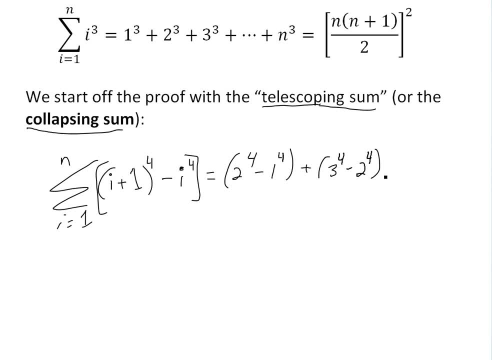 Now, since we have this here And as you keep going on, This would cancel, This would cancel, And then the next term is going to be well, 4 of 4 minus 3 of 4.. So then this would cancel, This would cancel. 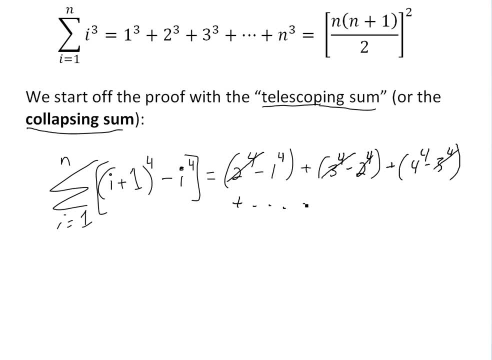 And you keep going on. The 4 is going to cancel Plus, etc. All the way up to well n. This is going to be n plus 1 to the 4. minus. This is going to be n to the 4 here. 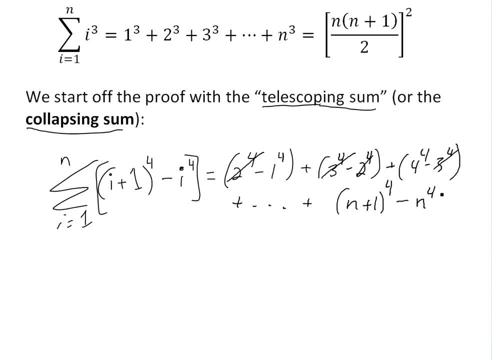 This is the last term here, And when you look at this order, You'll see that this will cancel out. Nothing is going to cancel out here, Because this one just cancels And you're going to have a 5. 5 to the 4 minus 4 to the 4.. 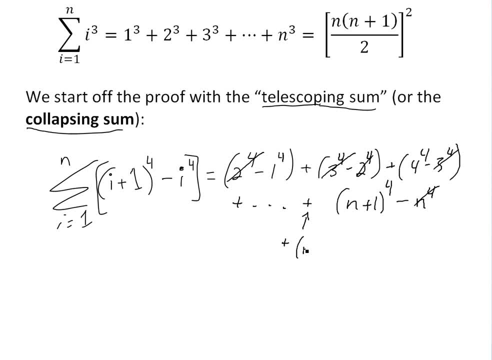 And the second last term here is going to be a plus n to the 4, minus n, minus 1 to the 4.. And then, So basically this would cancel with this And this one would cancel earlier, So it would have canceled earlier. 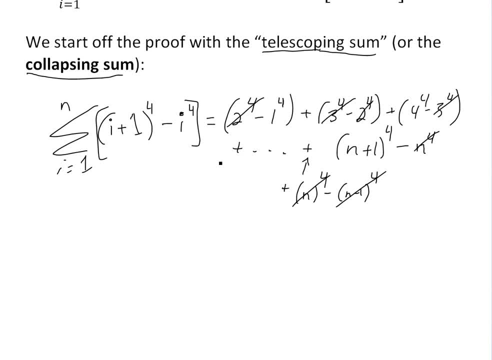 So this is. So we're left with just two stuff Because, as you can see, it collapsed into each other. So it's going to be n plus 1 to the power of 4, minus 1 to the power of 4.. Or just equals to well, n plus 1.. 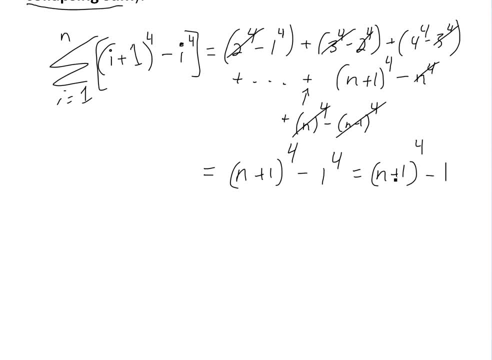 4 minus 1.. And to basically FOIL this out, You can use my FOIL method. Remember: this is just equal to n plus 1.. Well squared, And then the squared on top Negative 1.. So then the inside is going to be well. 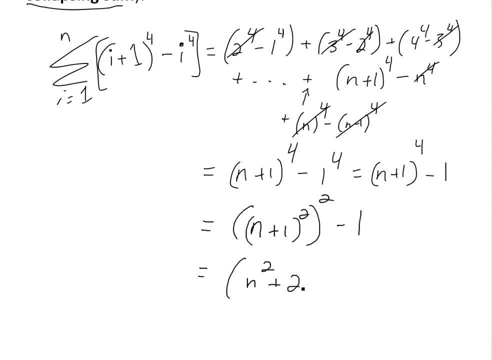 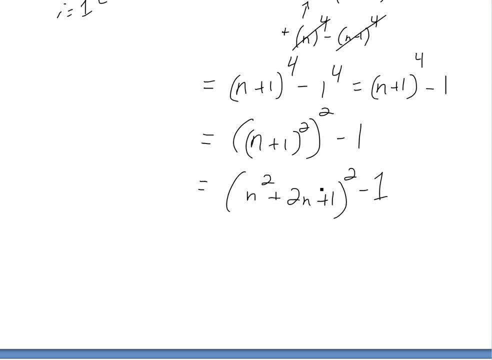 This is just going to be n squared If you FOIL out using the FOIL method 2n plus 1.. You can see the video link on the info below, Basically to see how the FOIL method, proof of it And also now you can do. 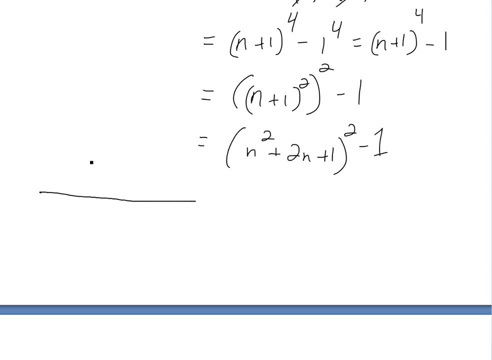 You can FOIL this out In a. Well, I have this quick method. You just make a table And you would just write down whatever, Because this isn't squared So this times by itself. So you write down each term on the top. 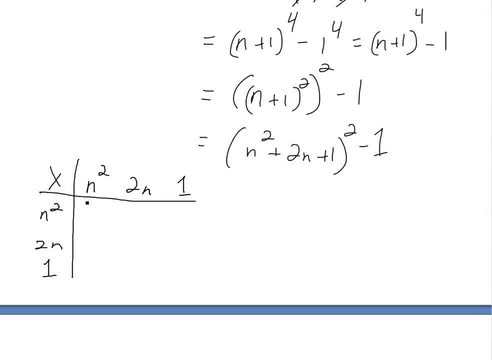 And on the bottom here, And then multiply each single column and row. This is going to be n to the 4. This times, this one here is going to be: This is going to be 2n cubed. This is going to be n squared. 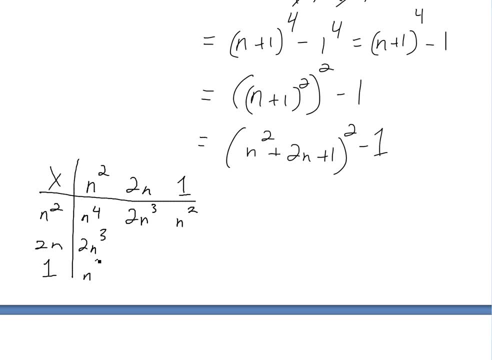 And this and this is going to be 2n cubed, This is going to be n squared, This is going to be 2n here, This is going to be 4n And this is going to be 2n squared. 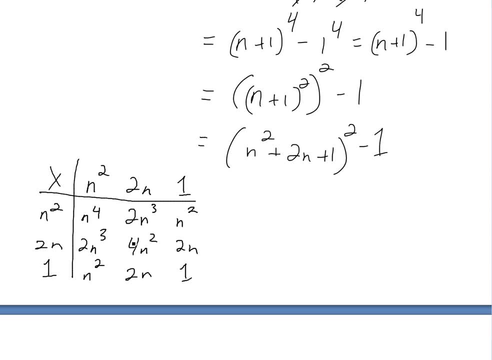 And now this is going to be 2n, This last one is going to be 1.. And then you just add them up on the diagonals, Because diagonals are the same: n cubed, n cubed, n squared, n squared, n squared. 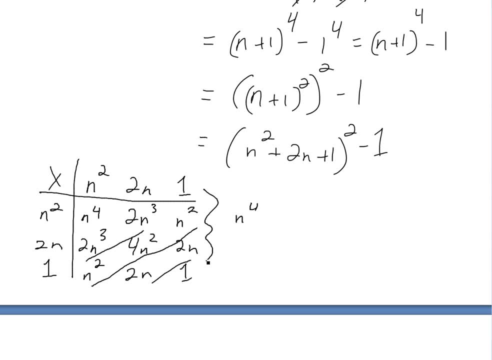 And n here. So you are going to get n to the 4.. The sum in this case, Or this term here, Is equal to Well, n to the 4.. Plus this one is going to be 4n cubed. 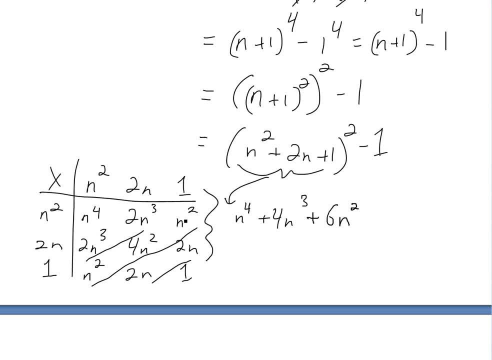 And then plus 6n, squared, Adding these diagonals, And then plus 4n, And then Plus a 1 here. So that is what this whole thing here, Or this n plus 1 to the power of 4, equals this. 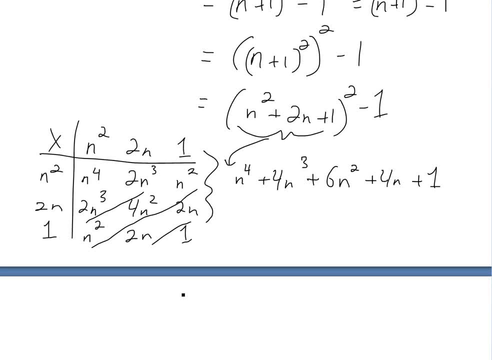 But then you have to subtract 1 to get the final formula. So then we just go equals. Well, that is summation. Yeah, the telescoping sum. in this case, This is going to be equal to n, to the 4. Plus 4n cubed. 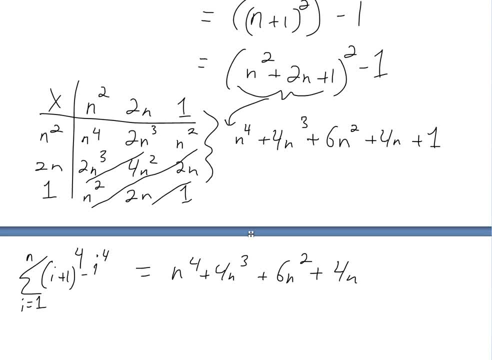 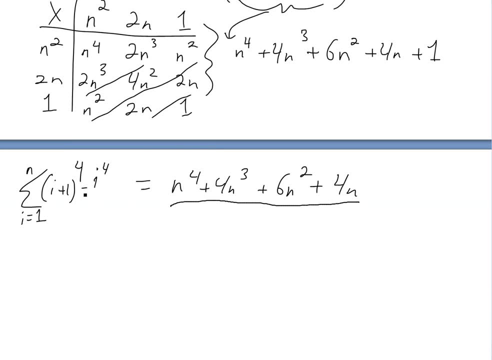 Plus 6n, squared plus 4n, And the 1s cancel. So we are left with this one here And now. I am going to show that, using Basically. we have this formula for this And we can also get a different formula. 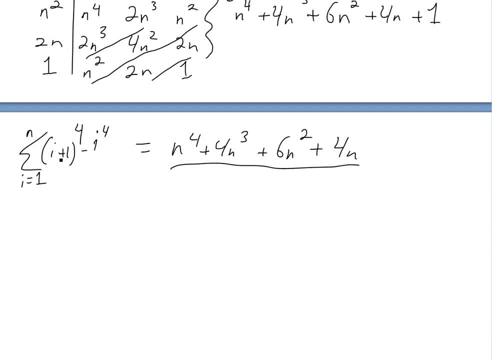 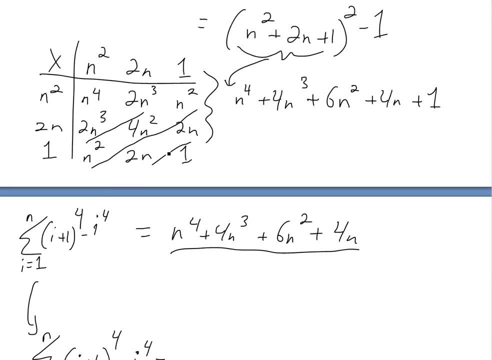 If we do a different method here, If we initially break this down, Factor it out first Or FOIL it out, Yeah, so if we FOIL this out, This one is exactly the same as n plus 1. But now we have an i there. 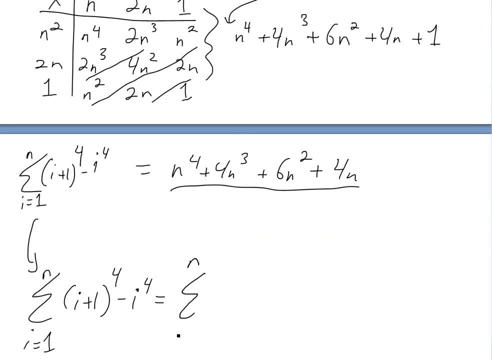 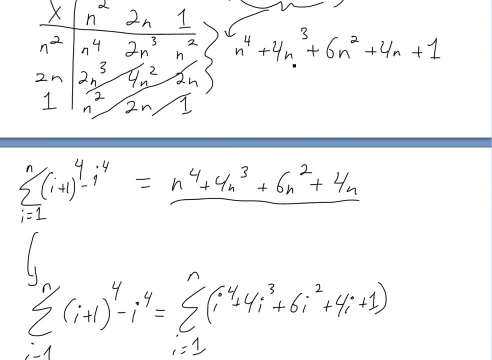 So we are going to get this one here Where you can just write that down. This is just equal to n, i equals 1.. Yeah, then we just write down. This is what we have here. This is FOILing out the n plus 1 to the power of 4.. 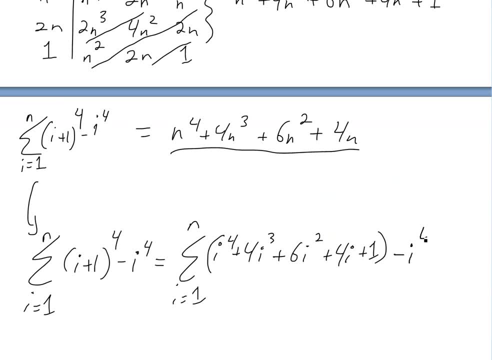 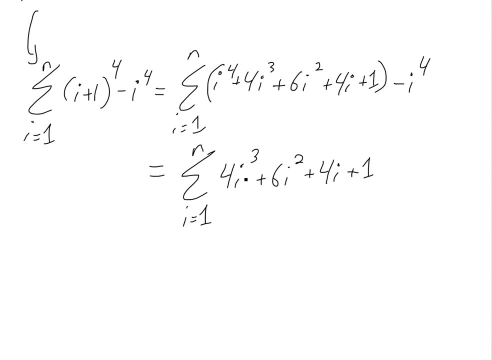 But this time we replace n with an i, Then we have to subtract the last part, The i, to the 4.. This one here, And then this would cancel. These would cancel. You are left with. Yeah, you are left with this function, right here. 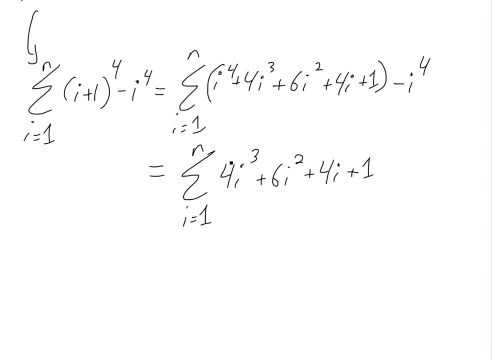 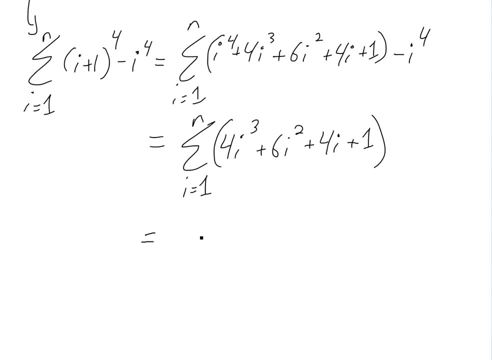 4i, cubed, 6i, squared, 4i and plus 1 here And now, if we use our The segmentation rules. You have seen the intro to segmentation. You can break this up into well separate summations. So this equals 2n i. 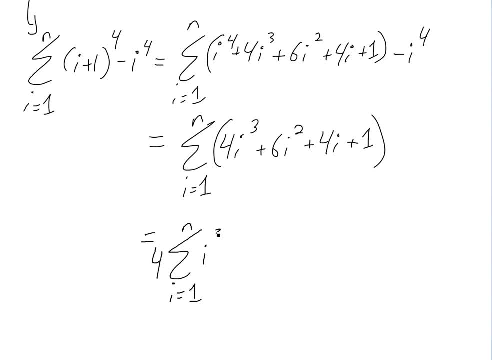 Equals 1.. Put the 4 out And then i cubed Plus take the 6 out. It is going to be: i squared i equals 1 of n, And then plus 4, sigma i equals 1.. And then the last one is just sigma 1. i equals 1 up to n here. 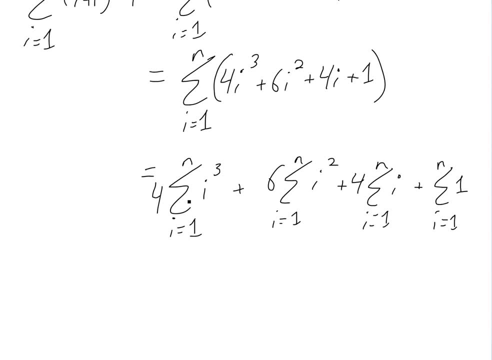 So now we have four different sums here. This one, we will just: This is what we want to solve, So we will call it 4s. So or just we will call this sum s that we want to solve. And now this one here: 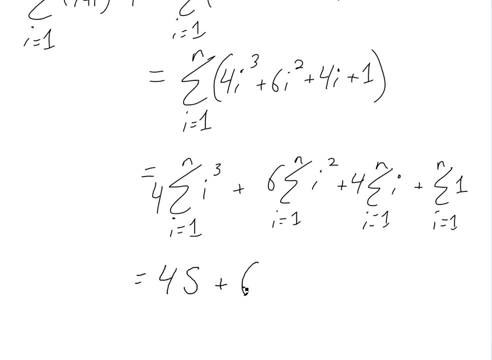 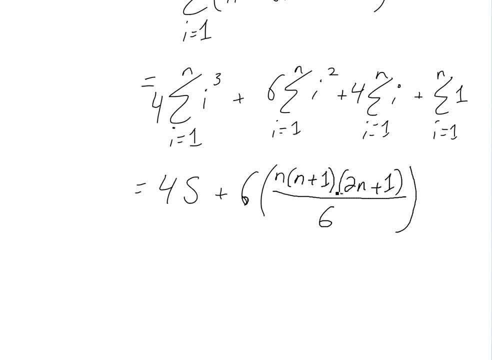 If you saw my other video, This just equals to well, 6 times the constant out Times. yeah, this one. the formula for this I showed in my earlier video on this is the sum of squares. It is going to be n times n plus 1.. 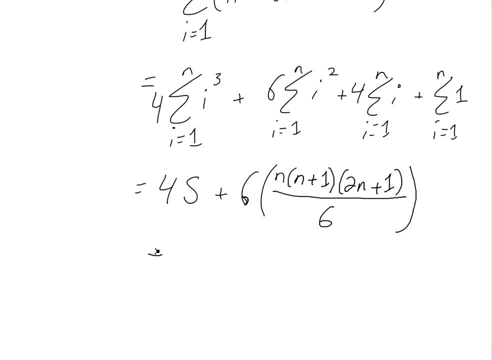 Times 2n plus 1 divided by 6.. And then, for this one here, Just the sum of consecutive integers. It is going to be 4 times. We have to plug in the formula for that And that is just going to be nn plus 1.. 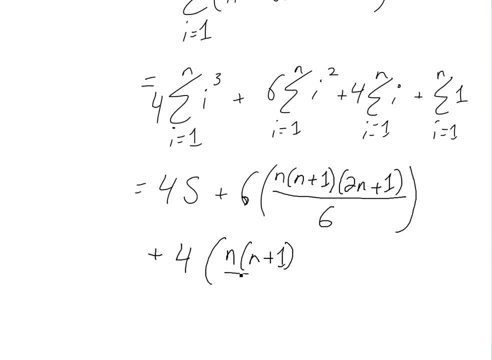 You can see the video link for the proof of this. And this one here divided by 2.. And then the last sum, This one here summing up 1, a million times. It is going to be 1 plus 1 plus 2.. 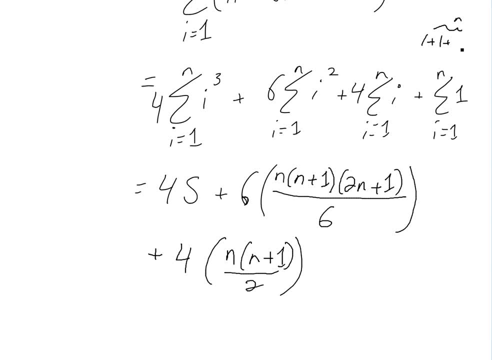 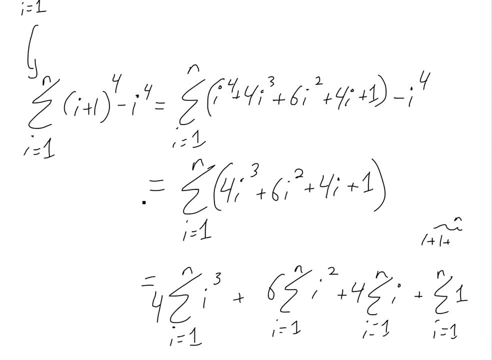 Plus 1, etcetera, up to n times, This is going to equal to n. Just summing up, that is basically what n is. So plus n here. So then we have two formulas For the telescoping sum, So this one and this one. 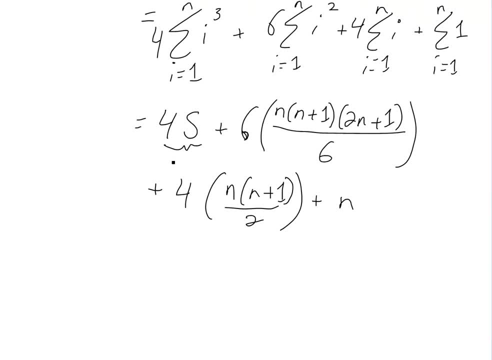 And this one has s. So all we do is equate them and solve for s. Well, before we do that, let us just simplify this side. First, it is going to be 4s, Then the 6s, cancel, And then plus. this times this inside. 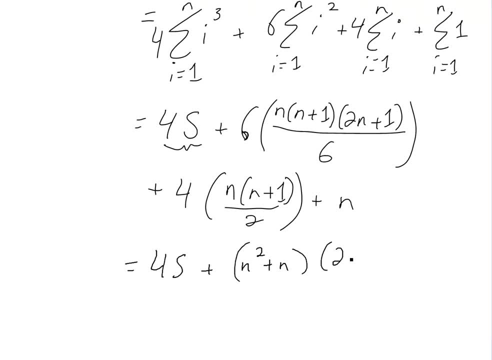 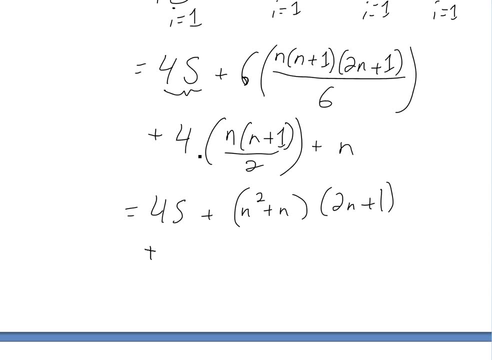 We are going to have n squared plus n, Times it by 2n plus 1.. And then all the way on this side here, This is going to be plus. This is a 2n now. This cancels and will be 2n. 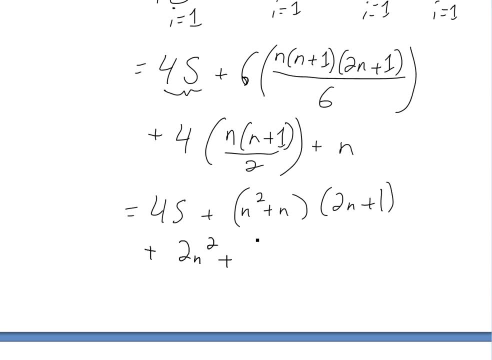 And multiply inside. So we are going to have 2n squared Plus 2n Plus n here, And n is from this one here And this one here. This is just multiplied 2n times n plus 1.. It is 2n squared plus 2n. 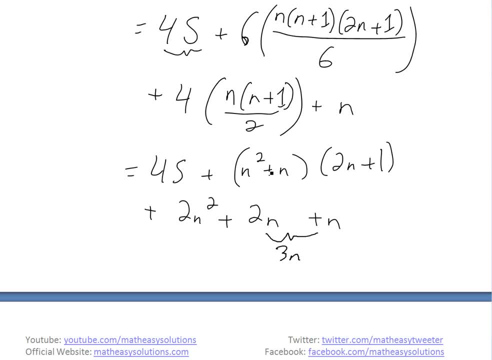 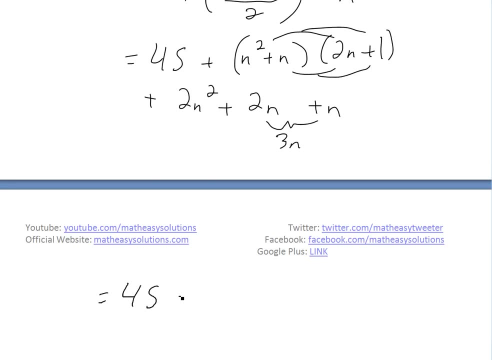 So now these two together is going to be 3n here. If we just simplify further, We are going to pull this out, Multiply this by this And this by this And add them up. You are going to get equals to 4s. 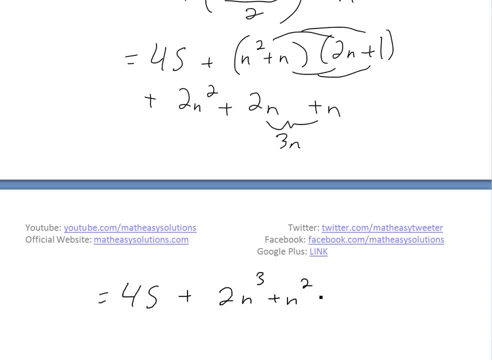 Plus, this is going to be 2n cubed, Just looking at it there- Plus n squared, Plus 2n squared, And then a plus a n here. So that is This times this plus this on this side here, And then plus. 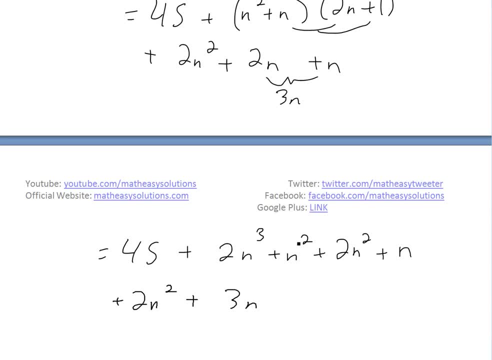 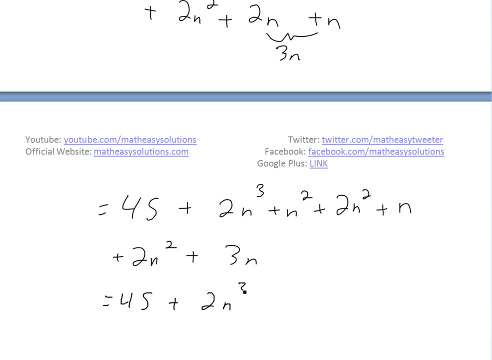 2n squared Plus 3n. And if we just simplify even further, here There is: We are going to have equals to 4s Plus 2n cubed. There is one cubed. Now there is three terms with n squared. 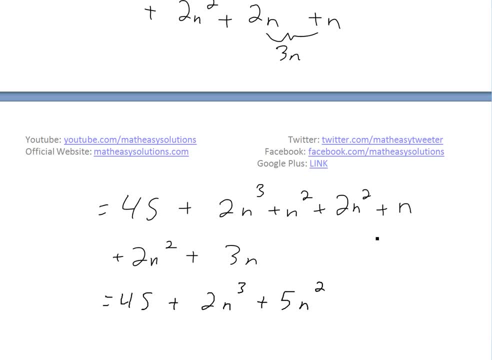 This is a. 2 plus 2 plus 1 is 5. Plus 5n squared. And then this one is n and n. This is going to be 4n. So now we just equate it with our first equation. 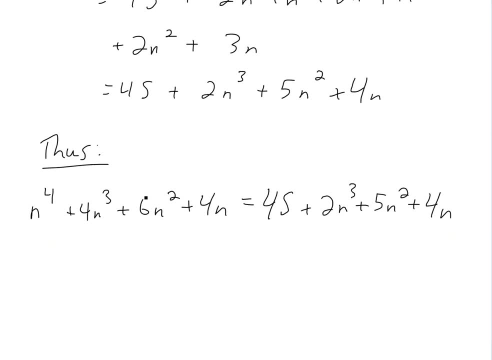 Which was this one here. Then, when we put this together here, This is the first equation we got, Using the telescoping sum, Just adding them up and seeing what happens, And then this is the one when we break them up apart Before we. 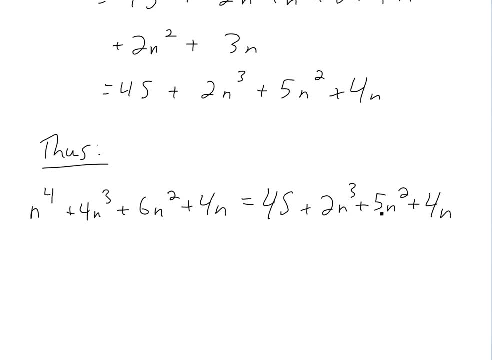 Yeah, we basically break them up And then we just write them in separate sums And, using the proofs- Proofs for the other sums, The squares and the consecutive integers- And we get this. So now we just solve for 4s here. 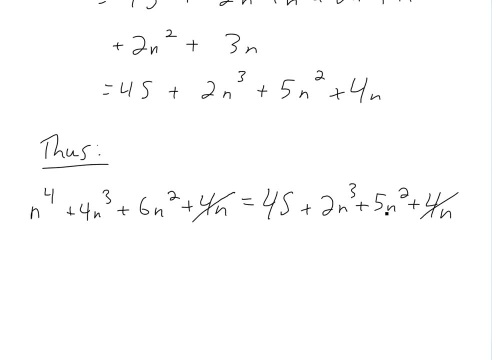 First we just cancel the like terms. This and this cancel here. Now, if we add up the, If we just take everything on the other side here, Make this one: here is a 5n squared. Now let's just write down what we can. 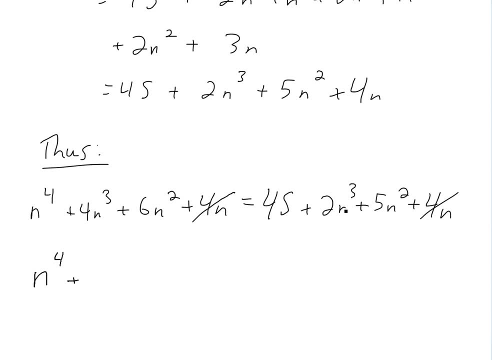 So n of the 4 is by itself Plus 4n cubed, Minus 2n cubed, This is going to be 2n cubed, And then this part right here: 6n squared minus 5n squared. 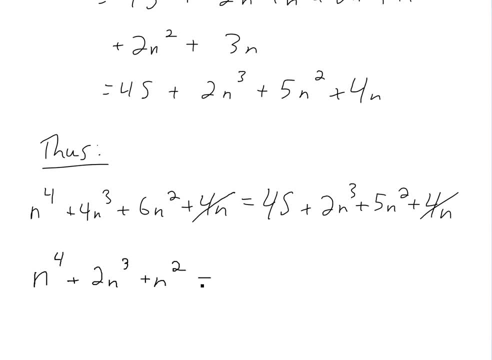 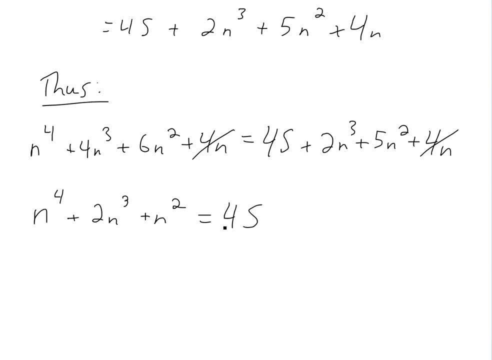 Is going to be n squared here, Other ones cancel. This is going to be 4s. So this is what 4s is equal to. Let's just break this up a bit more. And this one what we could do. 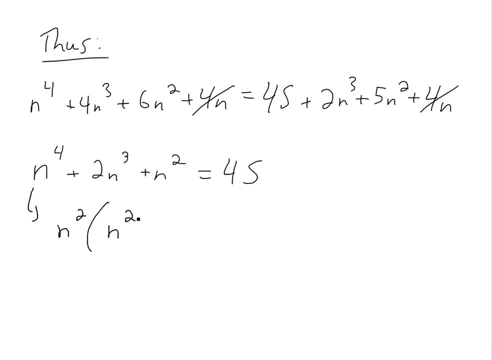 This part here. So if we take that n squared, We're going to have n squared Plus 2n plus This one is going to be a 1. Equals 4s And as you can see here This is a perfect square actually. 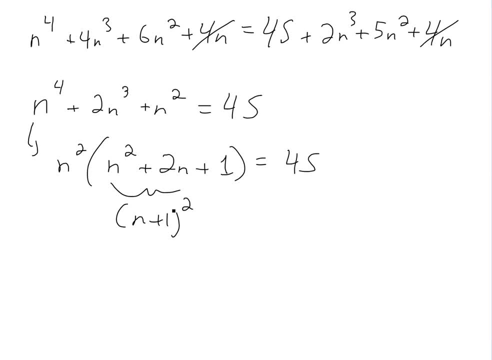 This one is just equal to n plus 1 squared, Because if you FOIL this out, This just equals to n squared plus 2n plus 1.. And that's this one, right here, If you FOIL it out. 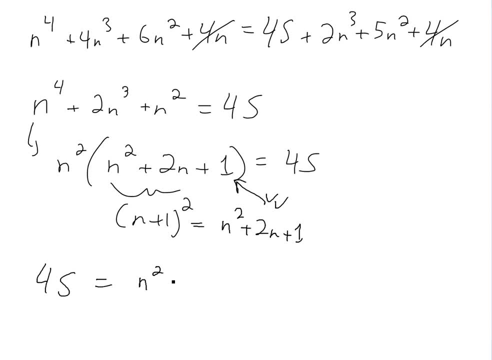 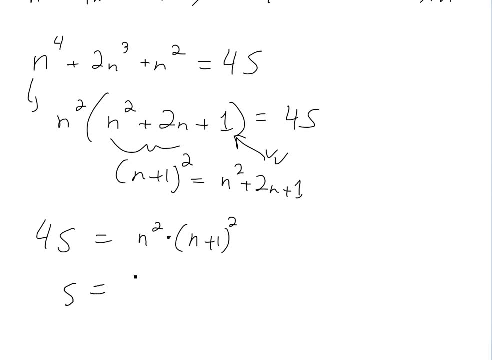 4s is equal to 4s is equal to n squared. times it by n plus 1 squared, And now we just divide out by 4.. So s is going to be n squared divided by n plus 1.. 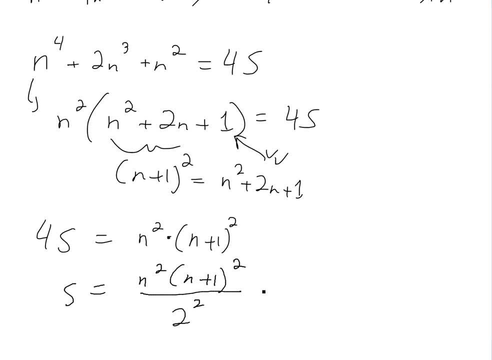 Now everything is squared. So let's just write the 4 as a 2 squared Instead of a 4.. And then we just take the squared out. So this is going to be n? n plus 1 divided by 2.. 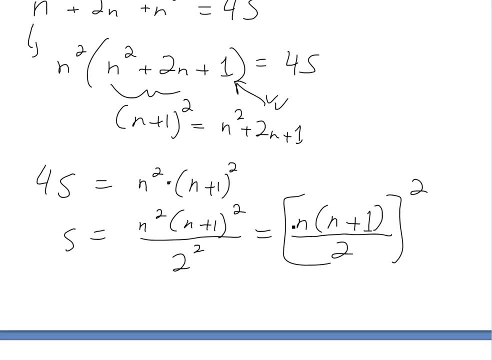 All squared And this is the sum of cubes, Of consecutive cubes, And this is the proof here. It's pretty abstract, Like the similar one to the squares one. You could do a similar one for, Instead of cubes, to the power of 4.. 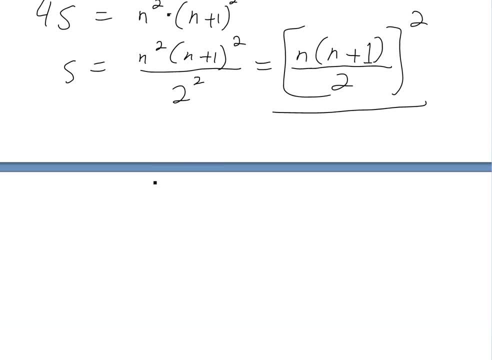 I think you could probably do it using the collapsing method As well. Well, now let's just do an example, Just to make sure at least we're getting it right here. So example: So if you look at this example, Where n is equal to 4.. 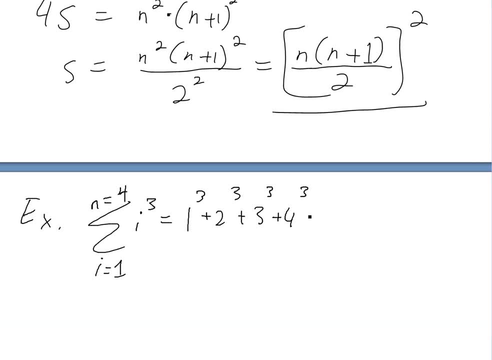 Plus 4 cubed. Then you could sum these up. Or let's just plug it into this formula above: This would just equal to: Well, n is 4 in this case, So 4 times. Now this is going to be a 5.. 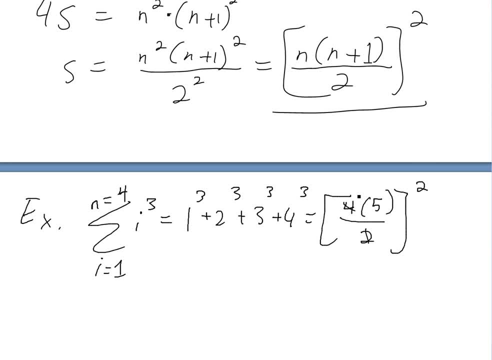 Divided by 2.. All squared here, And now this one here. as you can see, This just cancels. This is going to be a 2. And this 2 times 5 squared Is going to be 10 squared. 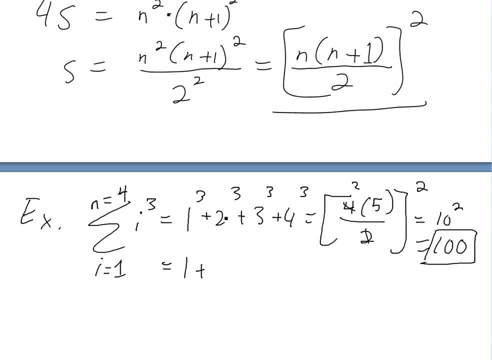 Just equals to 100.. Equal to well. 1 plus This is an 8.. And then 3 squared is And 3 cubed is going to be. Well, 3 times 3 is 9.. Times 3 is 27.. 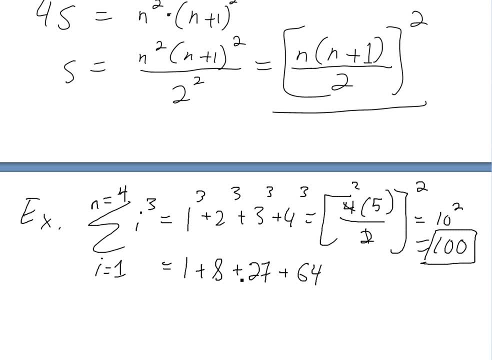 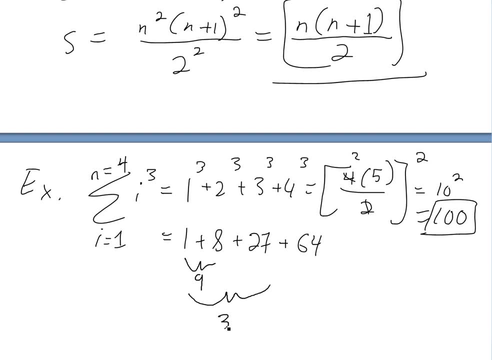 And then 4 times 4 is 16. And 16 times 4 is actually 64. So if you add these up Here, This is going to be a 9. And then, if you sum up these two here, This is going to be a 36.. 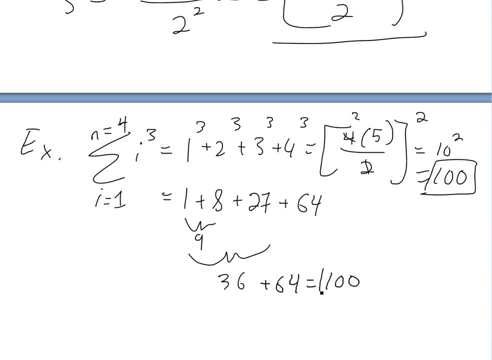 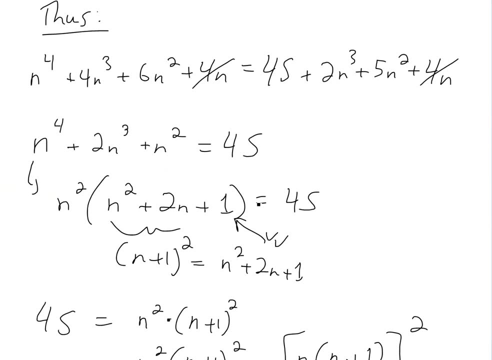 And then the last one here: 36 plus 64 is equal to 100.. So yeah, as I said, proof works. So yeah, that's all for today. I hope you learned. You can always download these notes In the drop box link below. 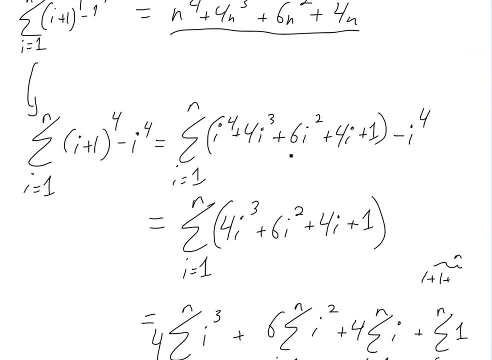 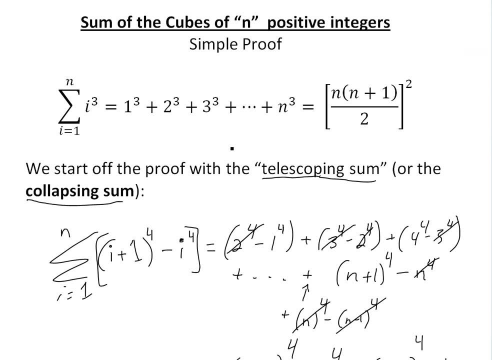 Let me know. if it doesn't work I'll fix it. But anyways, I hope you learned about this proof. It's similar to the sum of squares. You can see it in the video link below And also you see the proof for the. 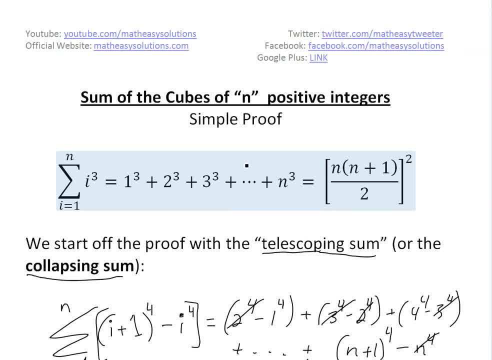 The other proof as well For the sum of squares And the consecutive numbers.